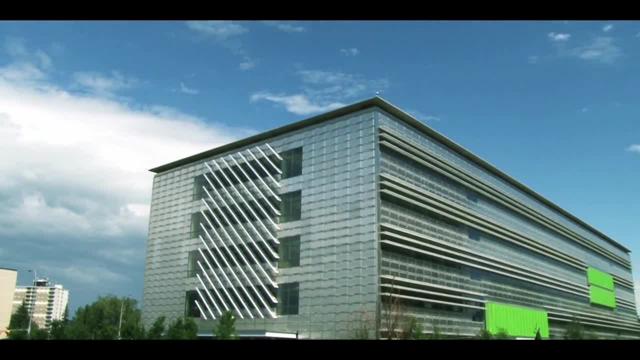 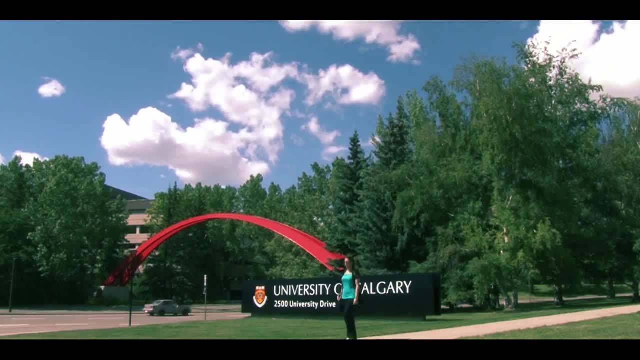 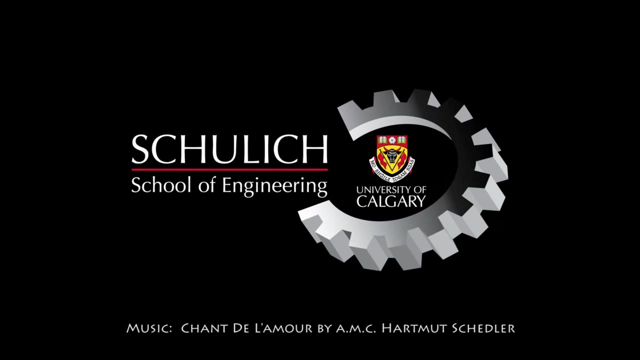 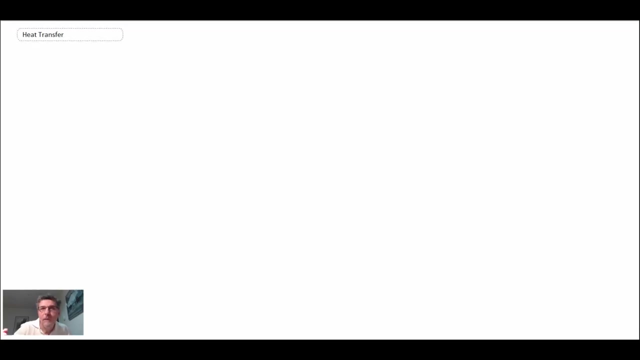 In the last segment. what we did is we came up with the idea of thermal resistances, and it is basically a bit of a shortcut technique for calculating conduction problems. So what we're going to do now? we're going to work an example problem involving thermal resistances and heat. 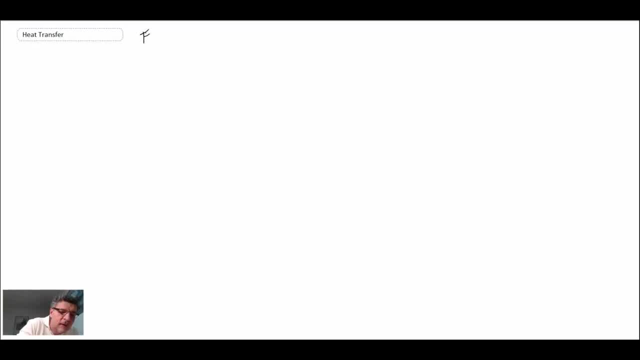 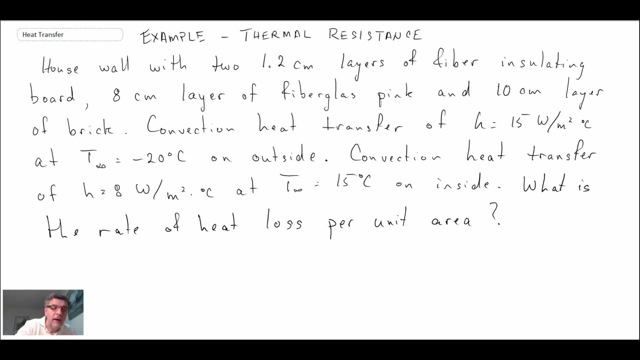 loss through the wall of a house. Okay, so there is our problem statement. What we have is we have a house wall that consists of two 1.2 centimeter layers of fiber insulating board and then there is eight centimeter layer of fiber. 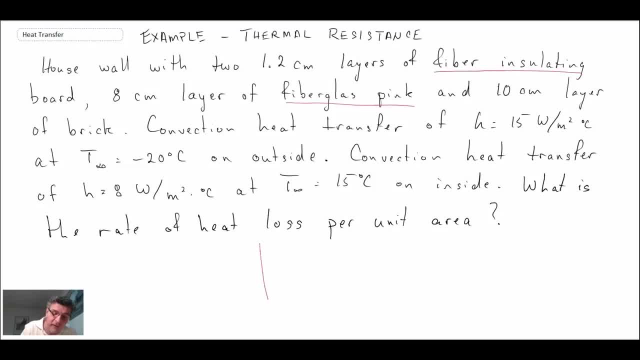 glass pink on the inside between those two walls. So we have a layer, a layer, and then inside, here we have fiberglass pink, And then what we have is we have a layer of brick on the outside, So there would be brick on the. 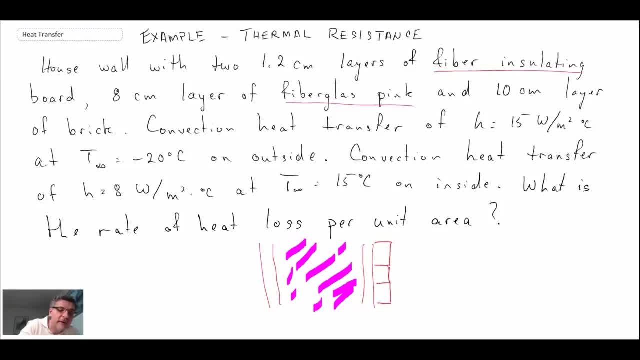 outside. And then what we're told is that we have convective environments on either side. So we have this layer of brick and then we have two convective environments. One is at minus 20- 20 degrees C, so that's pretty cold, and I assume that is on the outside of the brick. so the outside of the house, minus 20 degrees C- we have convective environment, we're told the convective heat transfer coefficient is 15 watts per square meter degrees C. and then we also have another environment on the inside of the house, and so you might have forced air heating or you could have radiators, but in any event you'll have air circulating inside of the house and the temperature. 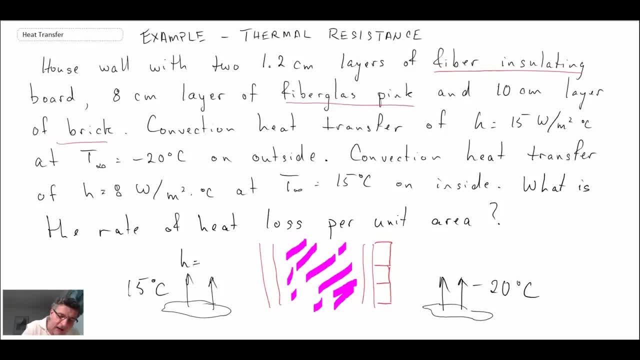 inside the house, we're told, is 15 degrees C and H is equal to 8, H outside was 15, so that is what we have for this problem. and now what we want to do. we want to be able to figure out what is the heat loss, the rate of heat loss through this system. and so you can see we're going: convection, conduction, conduction, conduction, conduction and then convection. so we've got a lot of stuff going on, but this is an ideal problem that you can use thermal resistances on. 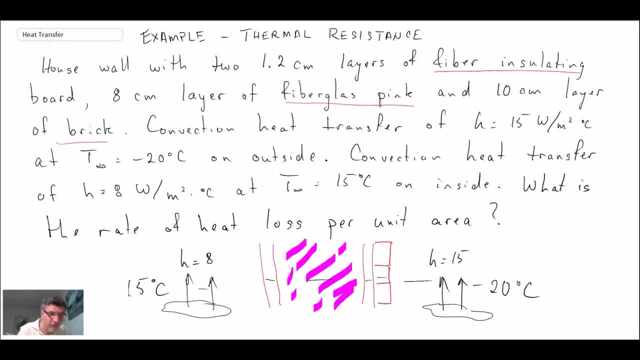 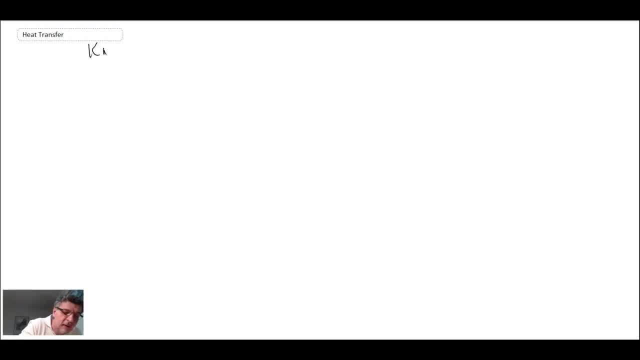 and it's a series problem, and, and so what we'll do? we'll work that and we'll begin like all the other problems. let's write out what we know, okay? so there is all the information that we were given in the problem. the last thing that 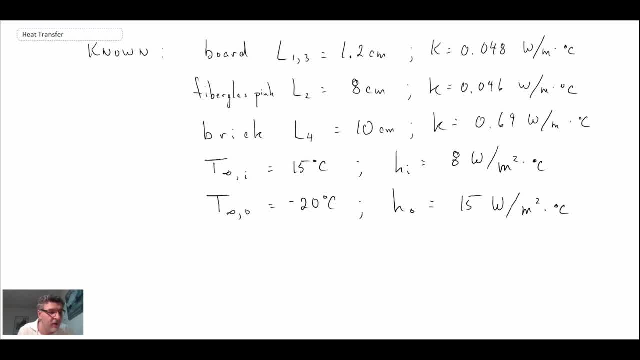 I'm going to write out. we were told to calculate heat loss per unit area and, consequently, what I'm going to do is I'm going to assign an area of one meter squared, so that is our unit area and the problem. we're looking for the rate of. 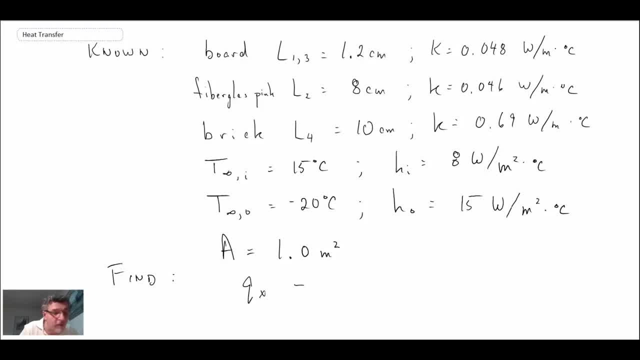 heat loss for the heat transfer rate. so we're going to assume this is one-dimensional and, looking at the problem, all of the assumptions that led up to the thermal resistance technique will work. you and those being: we have steady-state, one-dimensional conduction. there is no. 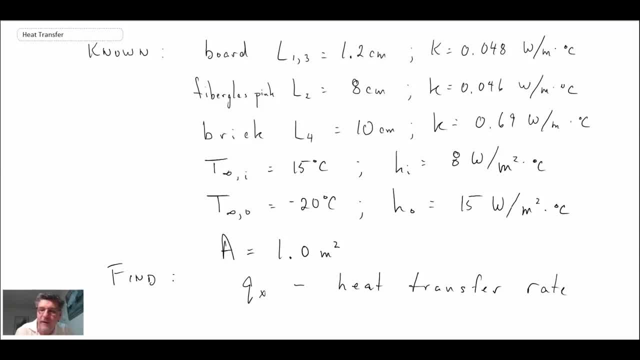 internal generation in the wall and the thermal conductivities will assume are not functions of temperature. so with that, what we'll do? we're going to come up with a schematic that has the coordinates and the information in terms of lengths and and things on it. so let me write that out. 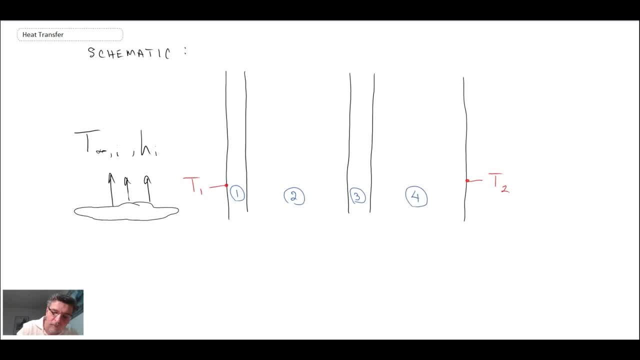 okay, so there is the schematic for our problem. we have the convective environments on either side and then the wall, and, just like I said earlier, we will assume the things that are required in order to apply thermal resistances, and that was steady-state, one-dimensional conduction, no internal heat generation, and the final thing is: 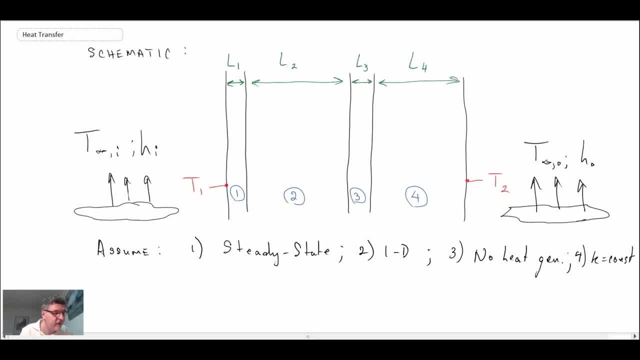 k is equal to constant for all the materials that we're dealing with. so, given that what we're now going to do, we're going to perform the analysis using thermal resistances, and this is a series problem, and so what we'll begin by doing is writing out what our resistance network looks like, and we're going to 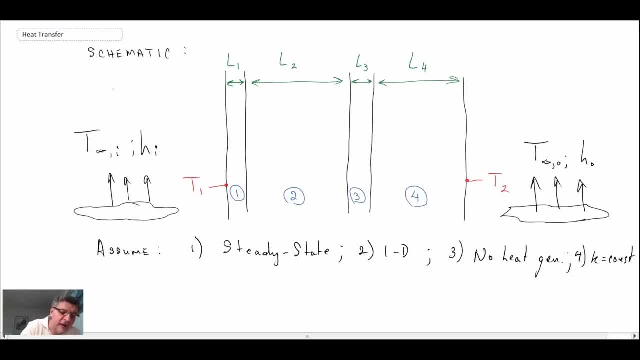 have the number of resistances that we're going to have. there will be one here, there will be two there, there will be three here, four, five and then finally, we're going to have six out here. that probably should have used different numbers, because that's going to mess this up with the widths. let me erase. 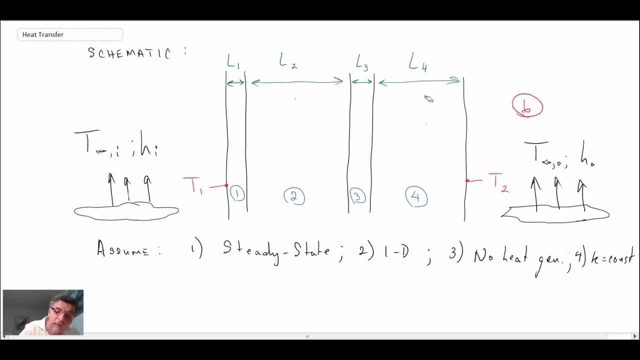 that. so for thermal resistances, I will do a, B, C, D, E and F. each of those is going to have a thermal resistance, although we're going to have a different symbol for it. but anyways, that shows you the number of thermal resistances. so let's. 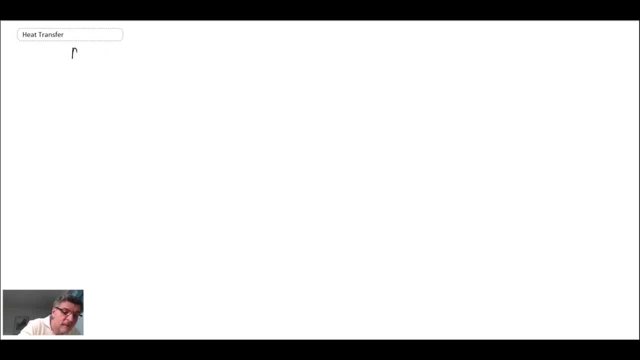 take a look at the analysis of this problem. so what we do when we're constructing our network, we begin with the temperature, that the one side, and that was T Infinity I- and then we move along and, and you'll notice, we first get to the convective environment, so that has a 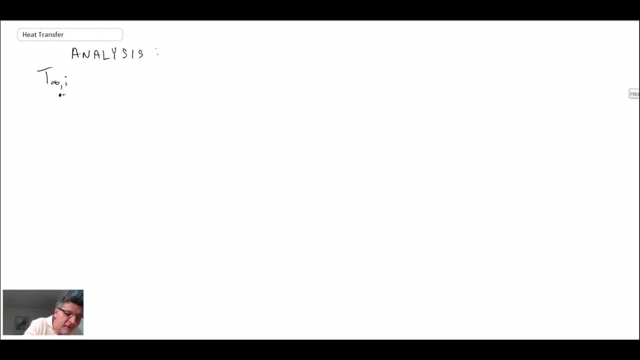 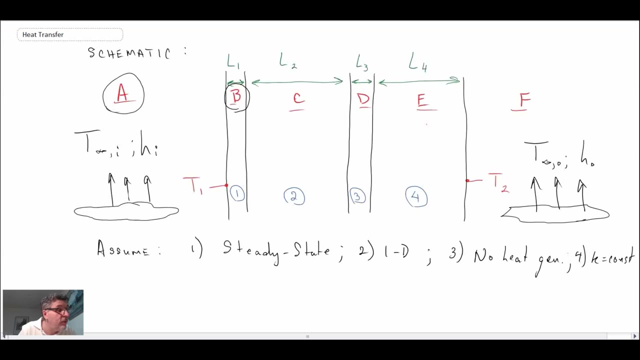 thermal resistance associated with it. so we put a thermal resistance and, and the val of that is going to be RT for thermal resistance, and then convection, and I'll do an I to denote that that is on the inside, and then we move along. looking back at our schematic, the next one that we hit is going to be the wall board. 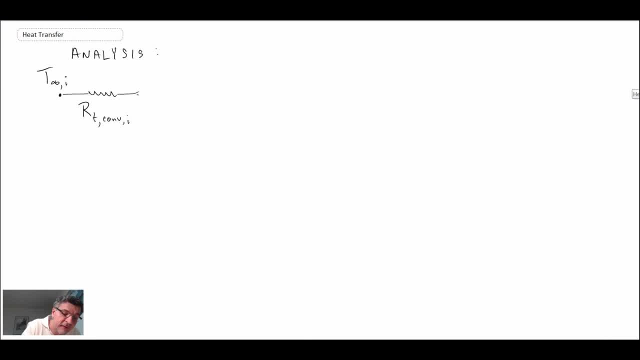 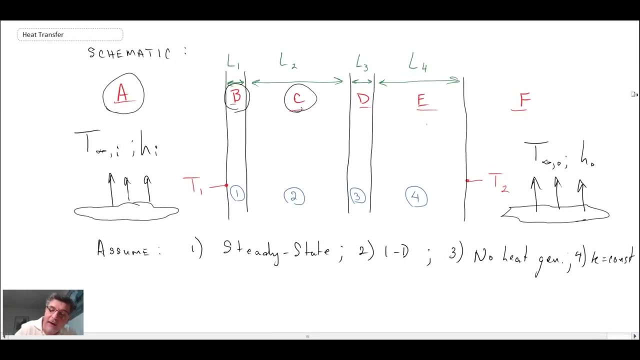 which is on the outside of the wall. so that will have another resistance and that will be due to conduction. so it will be thermal resistance conduction and I will give it the number one because that was the length scale that we had for that one. then we move into the fiberglass pink insulation and that 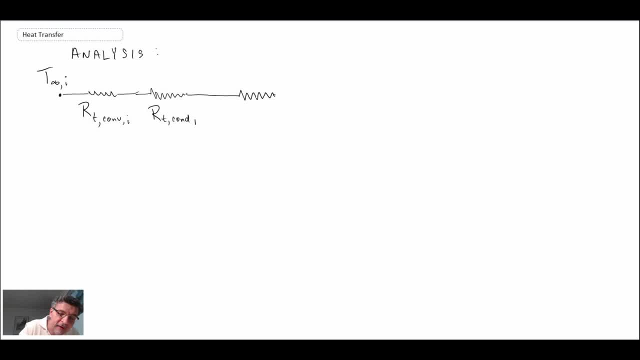 had length scale two, so that will have its own thermal resistance and that will be RT again due to conduction three. looking back at our schematic, we then go through another wall board length L3 and so that is going to have another thermal resistance, RT, conduction four. next one: we're going to have the brick which is on. 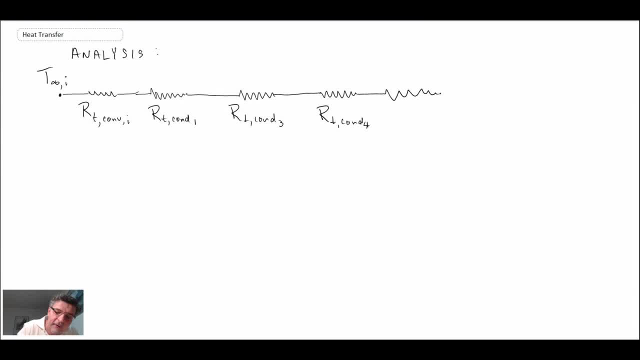 the outside of the wall, and so that is going to have another thermal resistance. again, it's going to be due to conduction, and that will be five. oops, sorry, sorry, I missed a number here. it should be one, two, three, four and then, finally, what we're going to have is the last one right here, that is, convective heat. 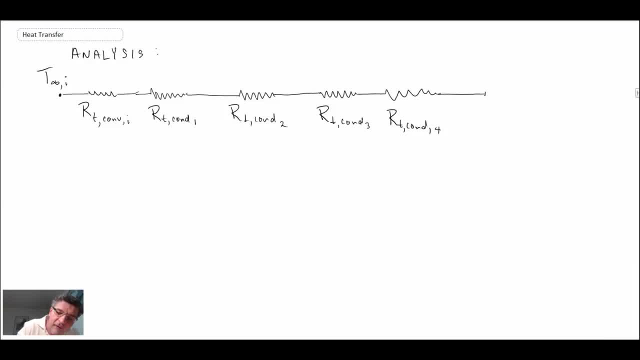 transfer. so we have a thermal resistance to end it here and that is due to convection and it is convective heat transfer on the outer surface. so I'll put a zero there and then finally, just like with the voltage, you have a voltage drop. here we have a change in. 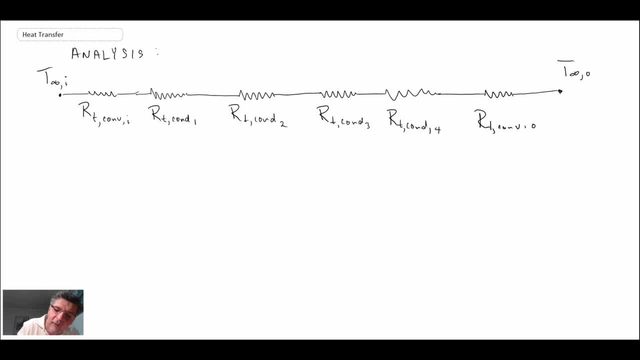 temperature and we're going to have a temperature drop and we then get to t Infinity outer. so that is our problem, or this scenario that we have, and now heat flux is going to be flowing in this direction and that is QX and that's what we're after. and the neat thing about thermal resistance is, although we're not, 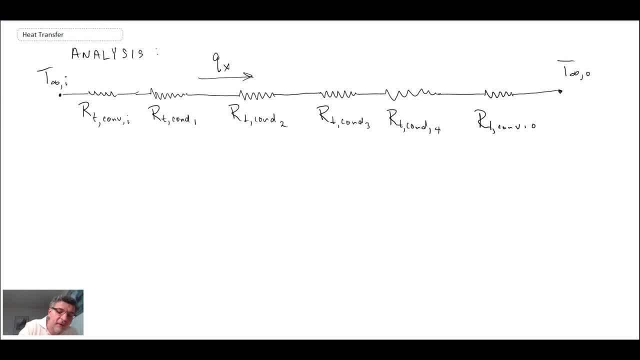 going to do it in this problem. once you solve Mr qx, you can use the equation for thermal resistances in order to figure out intermediate temperatures, And so that's kind of a quick way of computing temperatures at intermediate points. And you'll use the equation for the thermal resistance, basically the equivalent of Ohm's. 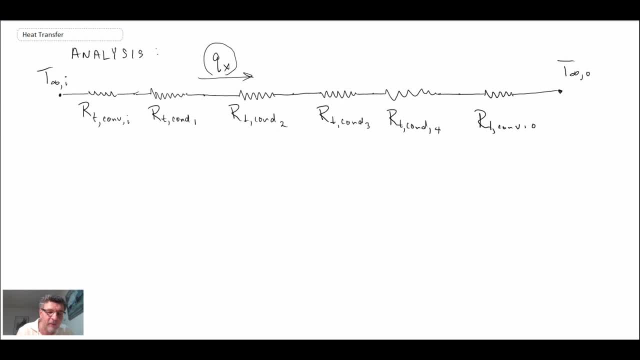 law that we have And that's how you could evaluate those which you would do. if you're doing electrical circuit analysis as well, You could calculate voltage at intermediate points. Well, here we can calculate temperature. So with that, what I'm going to do, I'm going to write out. 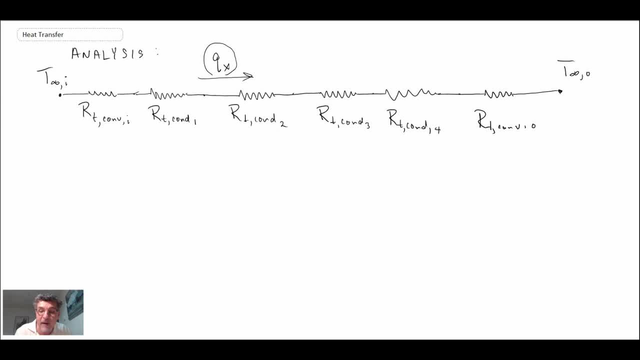 all of the different thermal resistances. We're going to sum them up because this is a series circuit, We'll put them in the equation and we'll solve for qx. Okay, so those are all of our thermal resistances. We're going to write out all of the different thermal resistances. 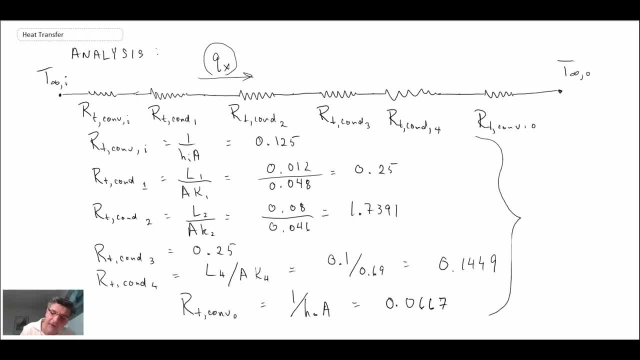 What I'm now going to do: I'm going to sum all of those, And so the total thermal resistance is going to be equal to sum of each individual component, because this is a series circuit And we get 2.5757.. And with that we can now put it into the equivalent of Ohm's law that we have. 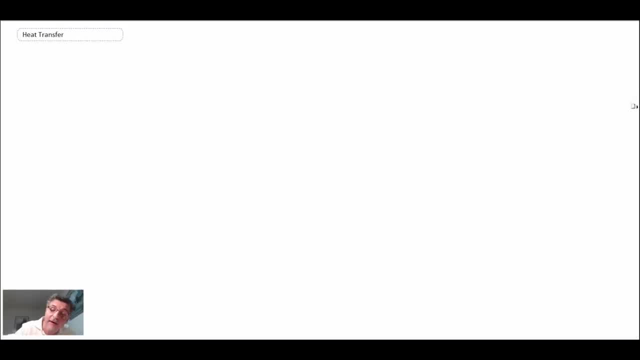 for thermal resistances. So let's do that on the next slide, And what we have then is qx is equal to- and it's going to be- the temperature change from one part of the circuit, from the start of the circuit, to the end of the circuit. So, looking back at our circuit, 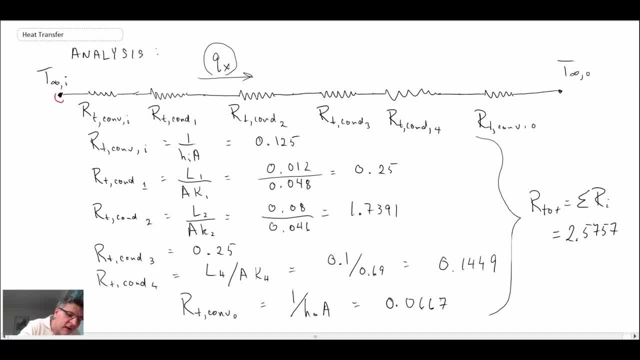 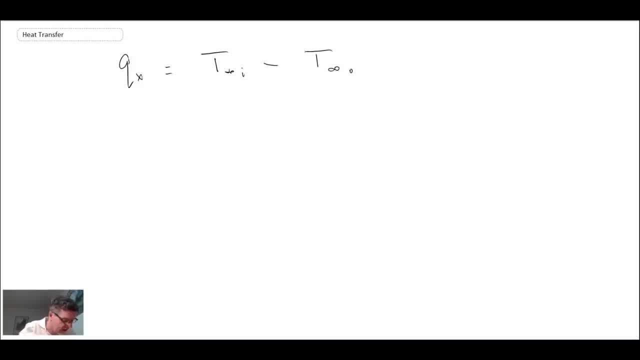 we're going from here- Let me do that in red- We're going from there to there. So that's going to be the temperature change over all of the resistances that we've computed, And when you do that, we'll divide by the total of the thermal resistance. 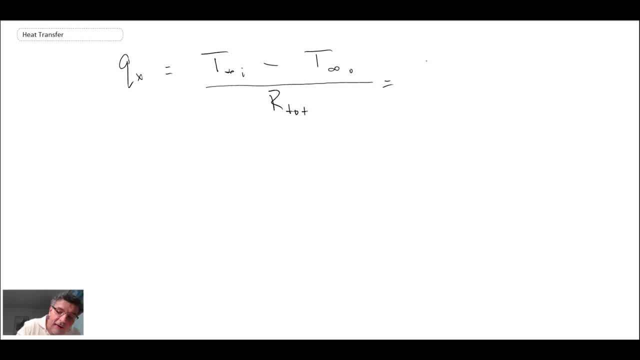 For all of the individual components And, if we recall, the inner temperature was 15 degrees C, the outer temperature was minus 20.. And then that's going to be divided by the sum of all of the resistances, which was 2.5757.. And with that we get qx is equal to 13.59 watts per meter. 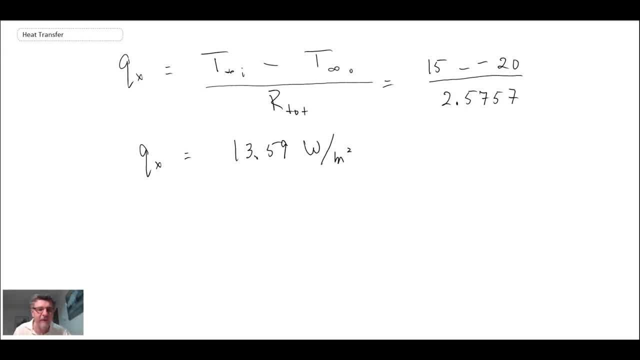 squared. And so there what we've done, we've calculated the thermal resistance And we've calculated the thermal resistance And we've calculated the thermal resistance And we've calculated heat loss through this wall using thermal resistances. It's quite a simple technique. 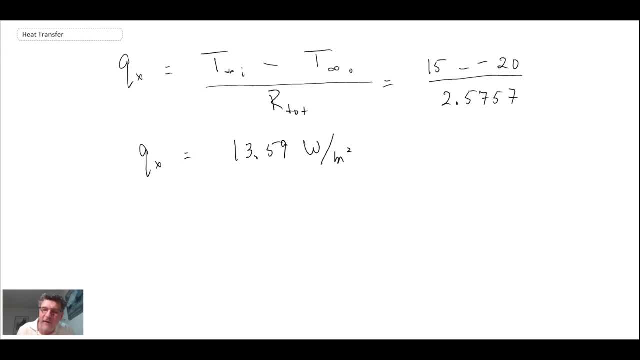 It's straightforward: You're just putting these resistance values together And, like I said, if you wanted to go in and evaluate the temperature at one of the intermediate points, you would just use this equation again, But the endpoints would change and the resistance values